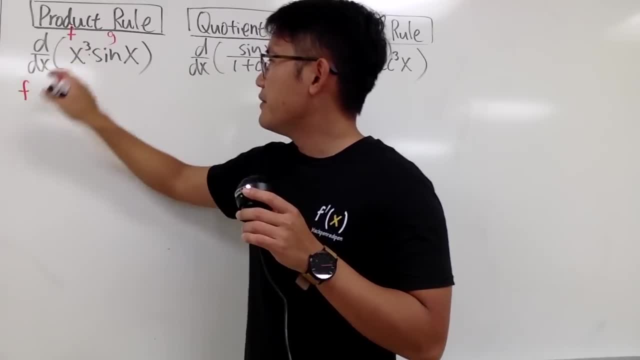 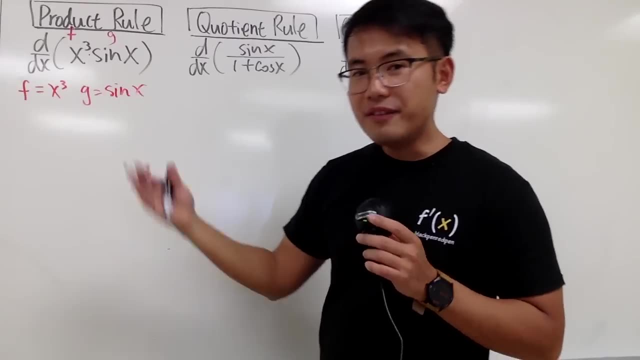 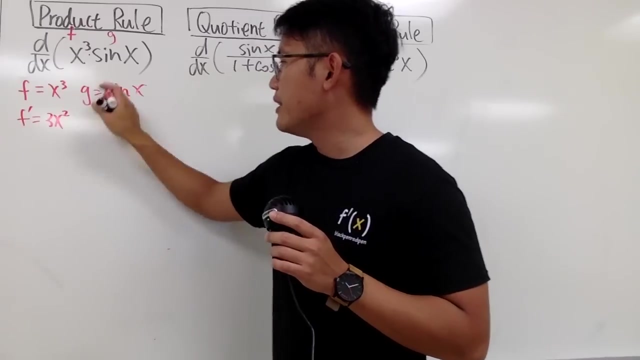 And I will write this down for you guys. to be more specific, f is x to the third power and g is sin x. And then from here I will just differentiate them individually: f prime, we get 3x squared, and then g prime, we get what's the derivative of sin x. 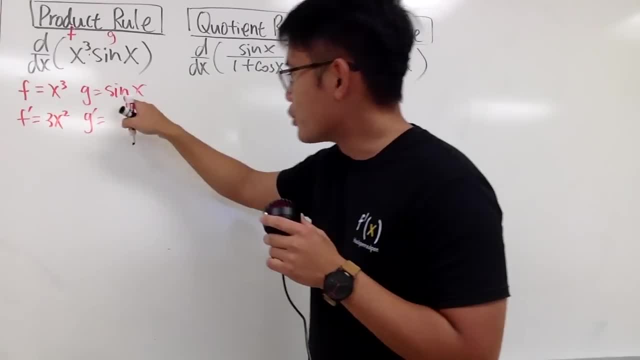 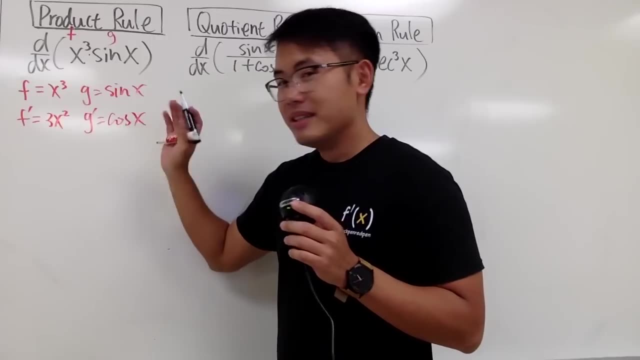 Hmm, This is something that you have to remember, okay, So the derivative of sin x is cosine x, okay, Yeah, Anyway, Now we have the ingredients and let me show you guys how to do the cooking Right here. 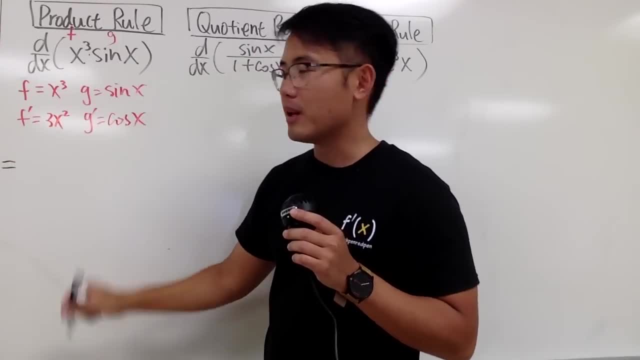 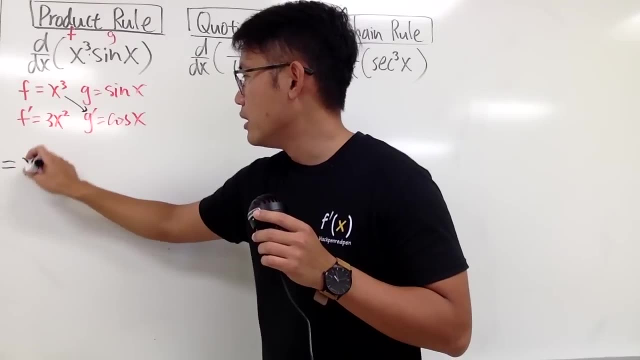 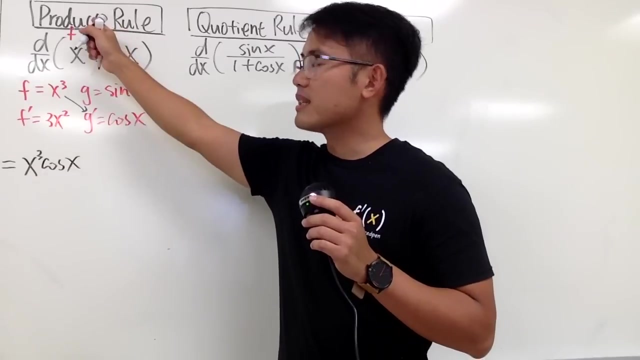 Here we will be able to construct our derivative by doing the following: You take this times that, namely x to the third power times cosine x. So let's put that down: x to the third power times cosine x. And then you have to remember you associate product with sum. 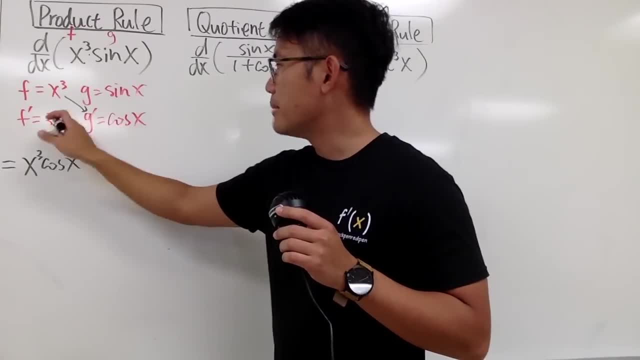 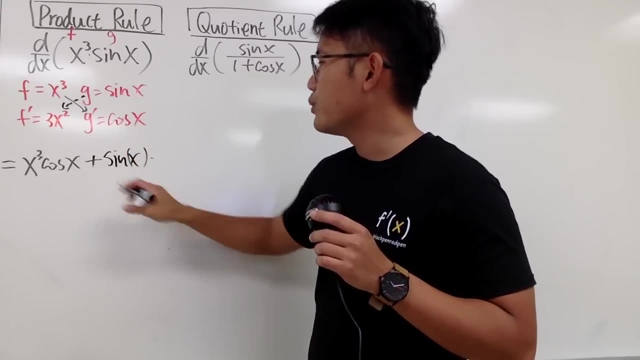 And you are going to add: okay, This times that then It's the other direction. I have sin x And let me put parentheses like this: And then we multiply by 3x, squared, okay, And that's pretty much it, okay. 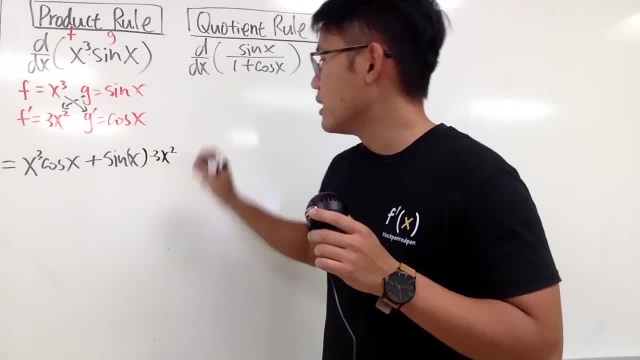 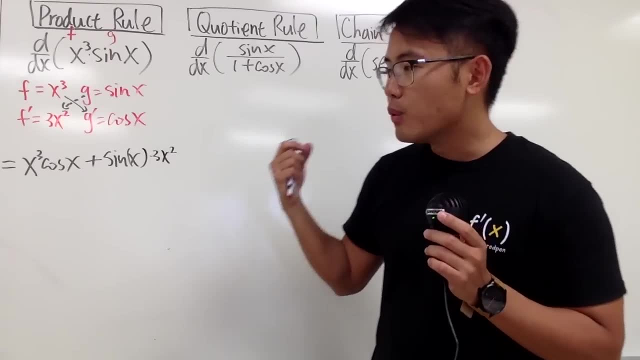 And, as I said, you can remember the formula And, in fact, you should be able to look at this and then put down this for the answer once. you practice this a lot, And that's the expectation, But, once again, if you are doing derivatives for the very first time, maybe memory devices will help. 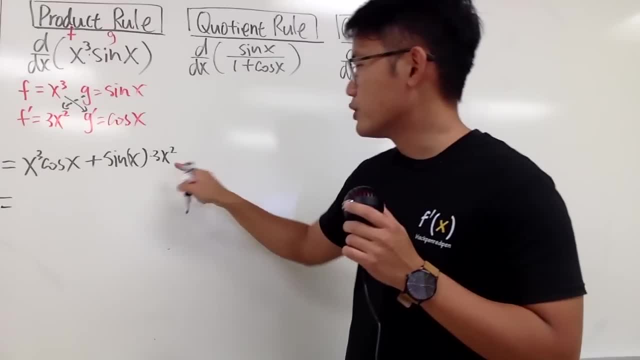 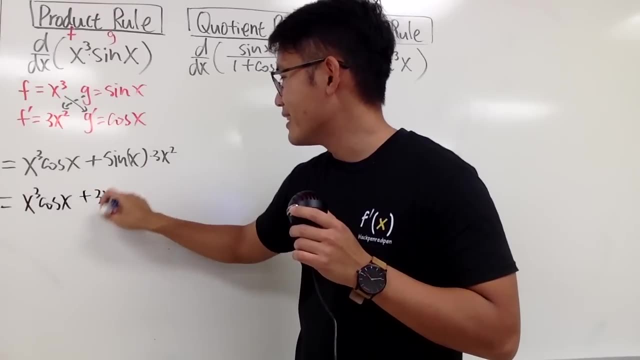 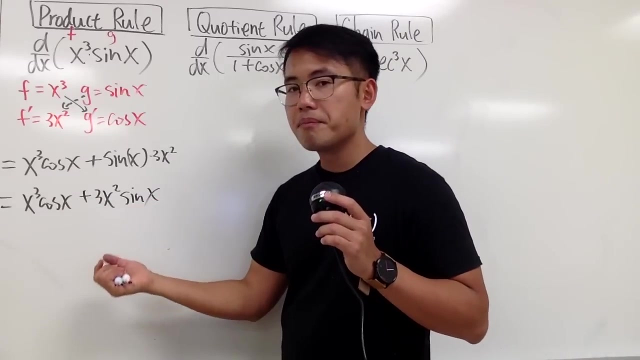 So give them a try. Anyway, in the end we pretty much just write this in the front, So we can write this down as x to the third power, cosine x plus 3x squared times sine x. And the usual deal is if you only have x inside of the sine or cosine, you don't have to put down the parentheses. 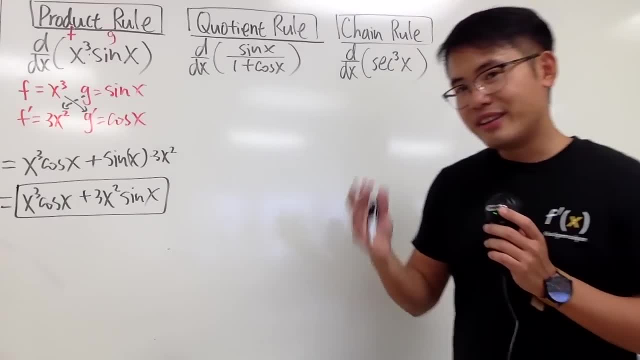 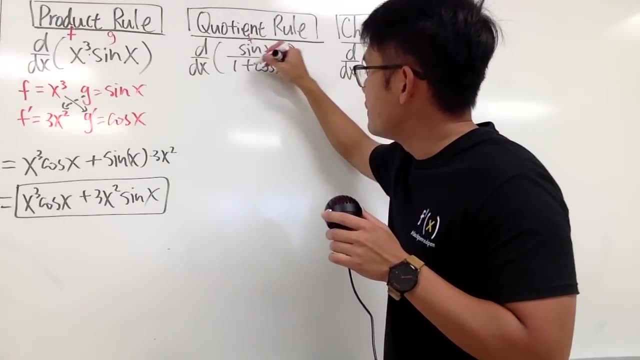 So this, right here is it for the first one. And now let me show you guys my memory device for the quotient rule. On the top, I will label this to be f. On the bottom, I will label that to be g. 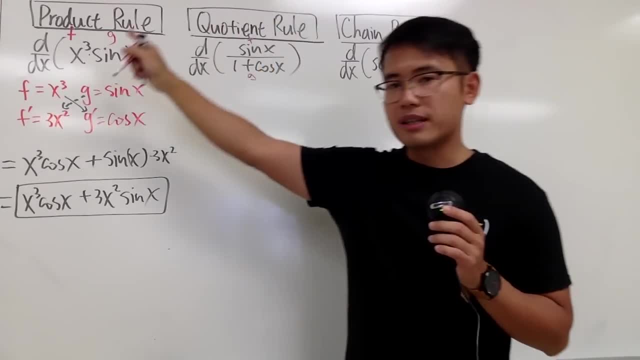 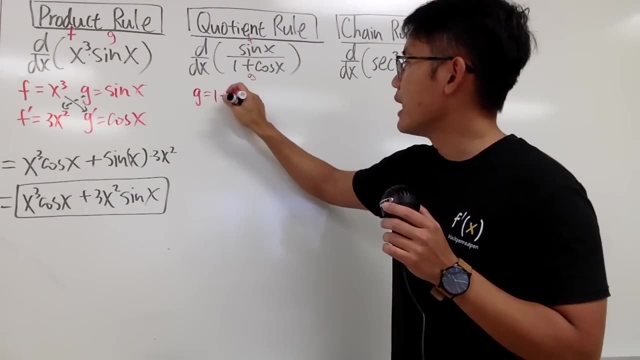 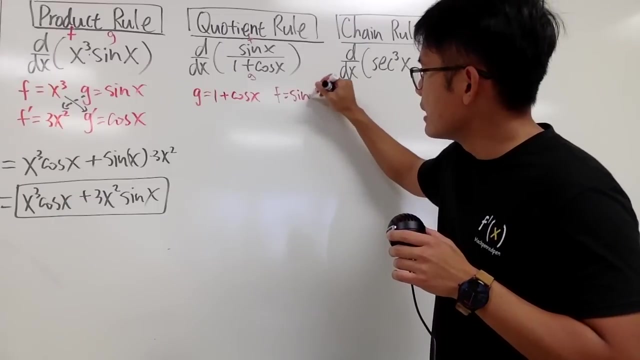 But you have to remember quotient is the upper And on the bottom I will label that to be f. So in this situation I will have to write down g first, which is 1 plus cosine x, And then on the side we put down f, which is sine x. 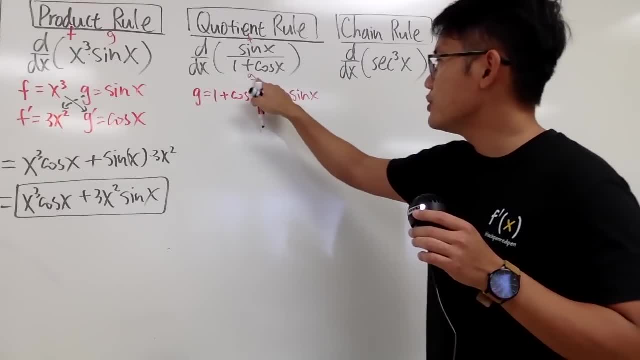 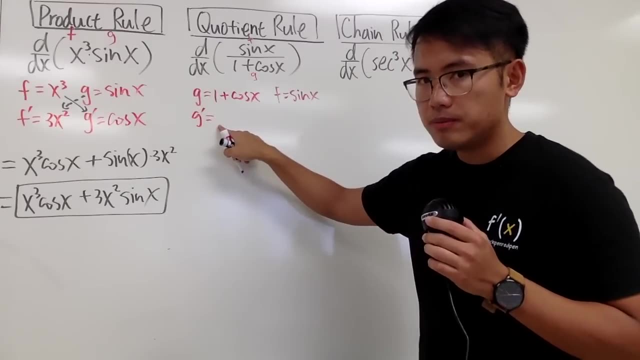 Write them down so that you can just differentiate them individually. So right here, g prime. The derivative of 1 is 0.. The derivative of cosine x is negative sine x. The derivative of cosine x is negative sine x. The derivative of sine x is negative sine x. 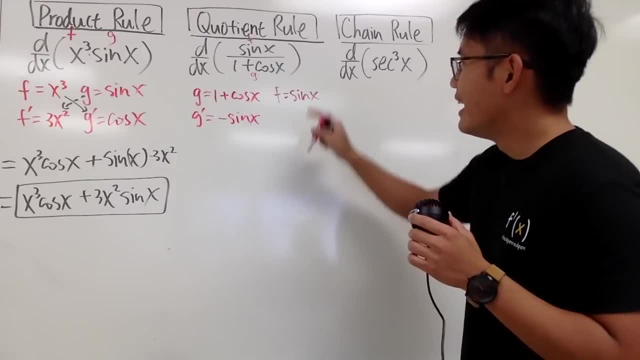 And, once again, this is something that you have to remember, And, once again, this is something that you have to remember. And right here, differentiate sine x, we get cosine x. And right here, differentiate sine x, we get cosine x. 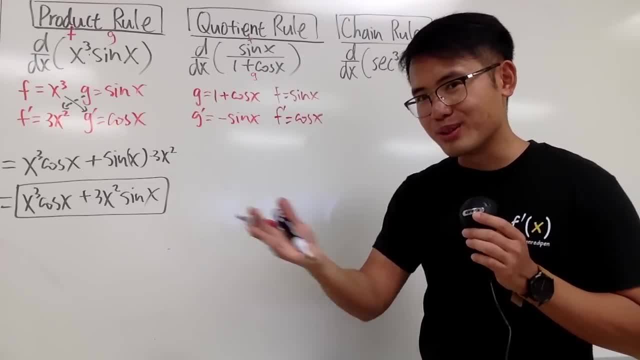 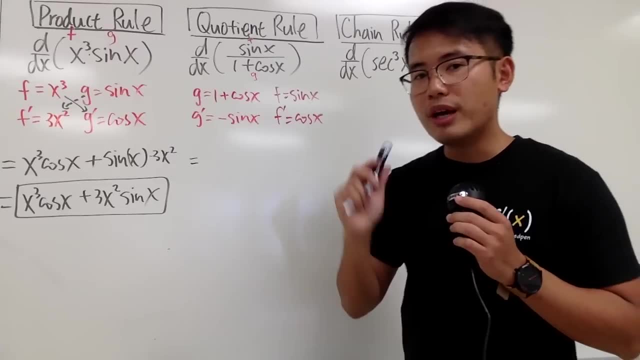 And now these are the ingredients. I will show you, guys, how to do the cooking Well in this situation. remember: if you start with a fraction, you are going to end up with a fraction, most likely, So go ahead and draw that fraction bar. 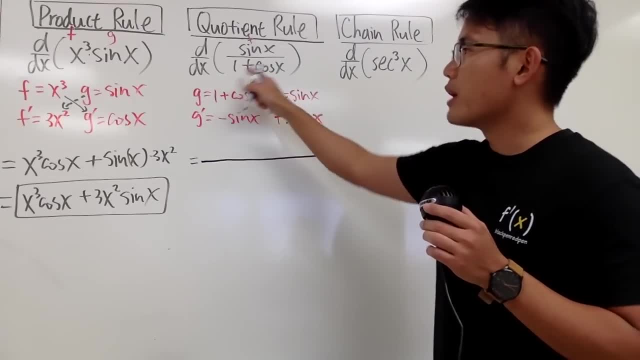 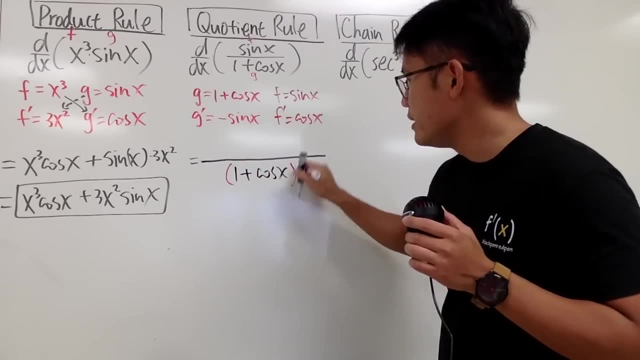 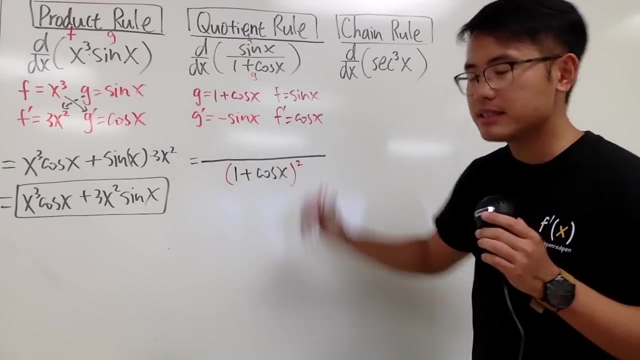 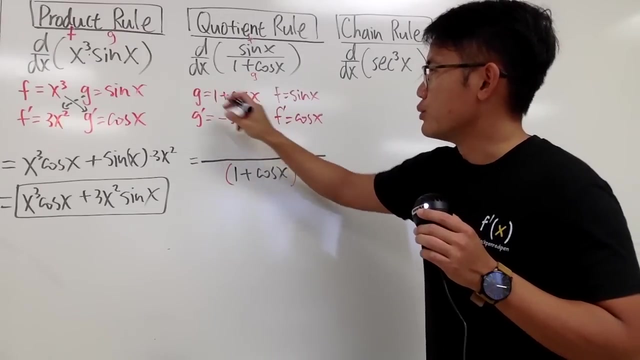 And before you do anything, go ahead and square the denominator. put this down: one plus cosine x, and then you are going to square the denominator like that, and then for the top, this is where we are going to use this memory device. i will go this times that, okay, still pretty much the same thing. well, this right here has two. 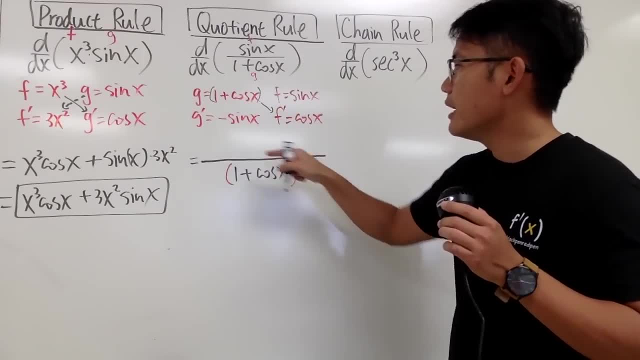 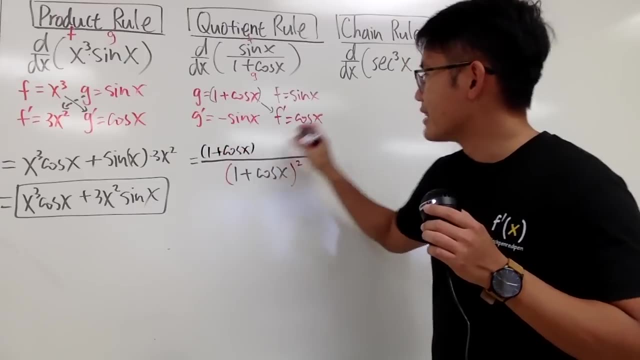 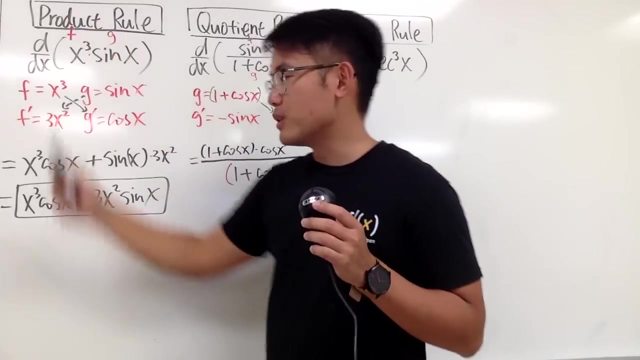 terms. so be sure you put down parentheses and then you multiply this and that and that goes right here. so that's one plus cosine x and then times this cosine x. and remember earlier i told you you associate product with sum right? this time you are going to associate. let me just make it. 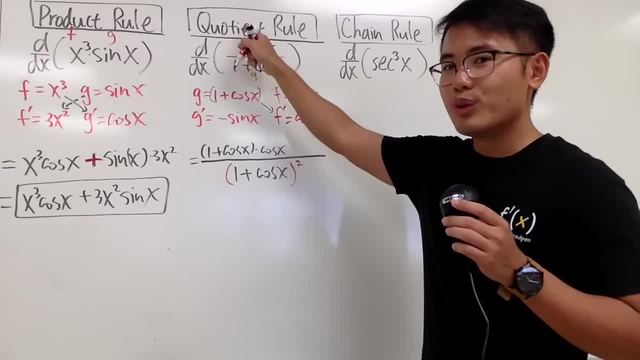 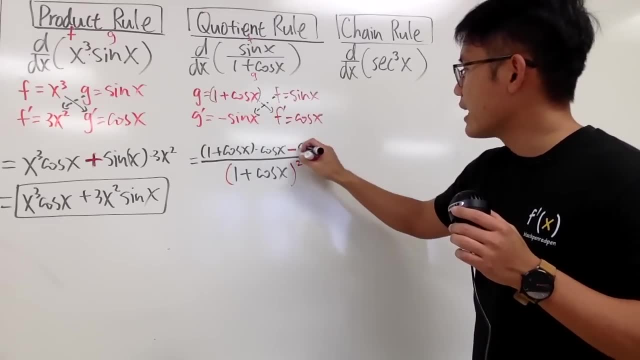 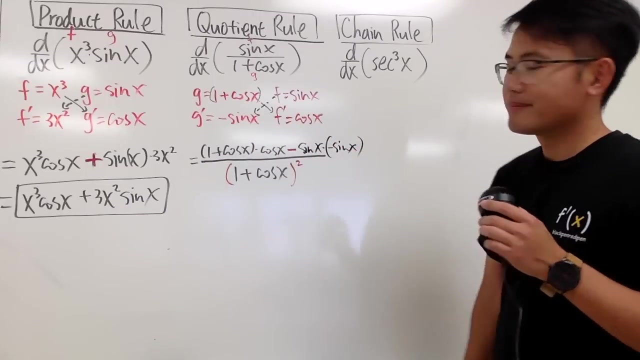 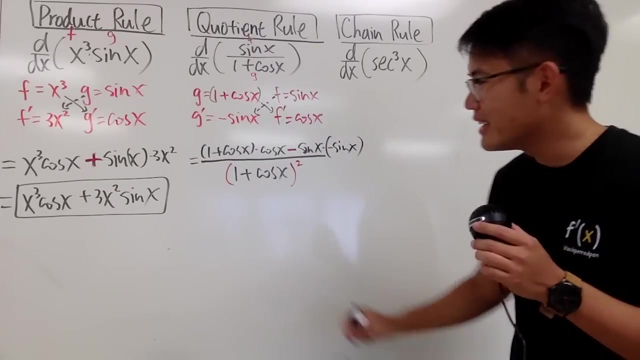 better. this time you're going to associate quotient with subtraction, so you're going to subtract this times. that then okay, so we have this sine x, and then i'm going to multiply by this negative sine x, like that. okay, from here, this is pretty much it. the rest is just: you do the identities, you just combine terms forever. okay, so we'll see. 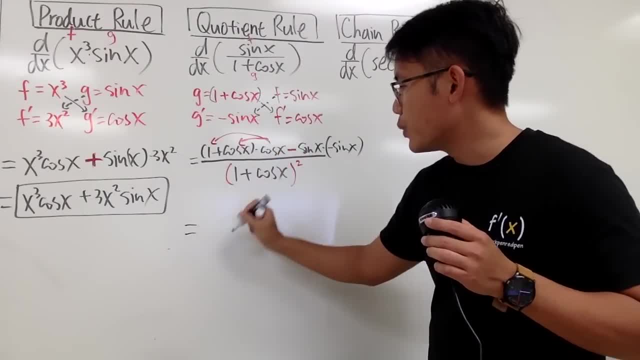 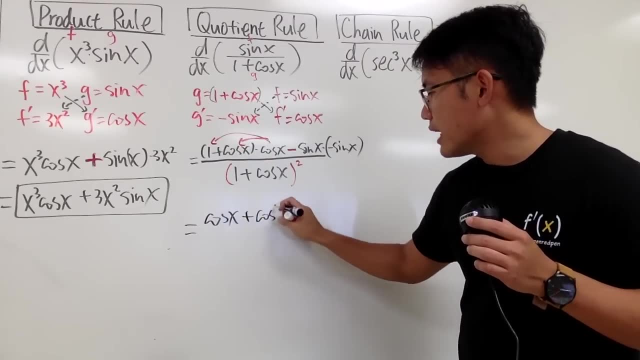 you can distribute this, of course, on the top. here we have cosine x times one, that's cosine x, cosine x times cosine x, that's plus cosine square x, and then this times, this negative times negative, becomes cosine x, and then you can distribute this, of course, on the top. here we have cosine x times. 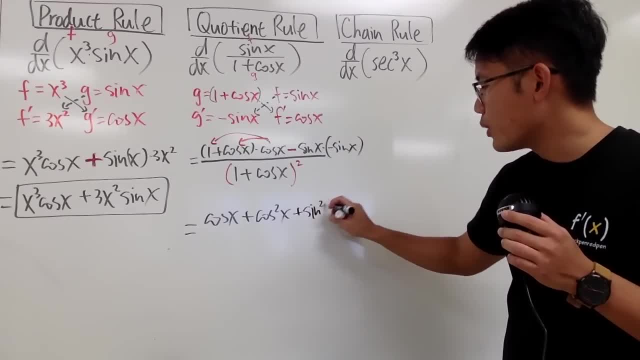 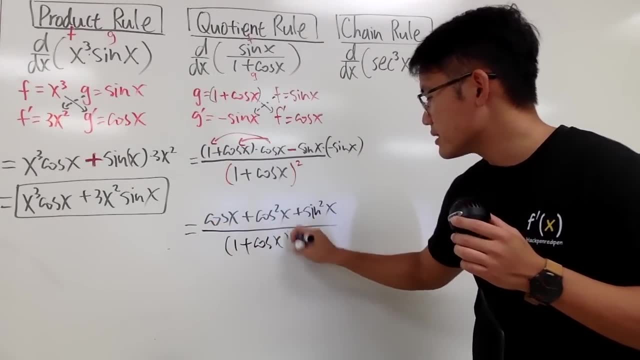 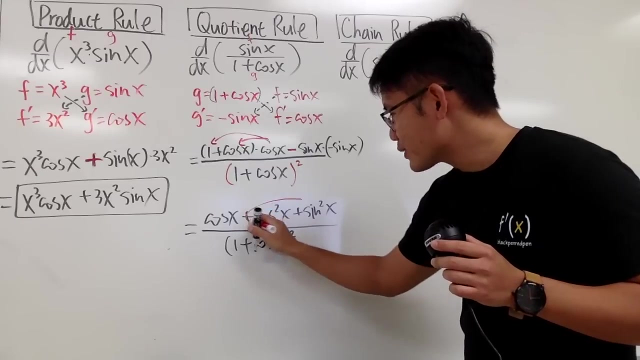 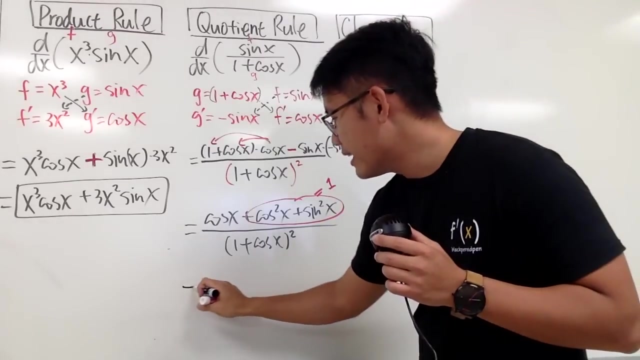 plus sine x times x, that's sine square x. and then on the denominator we have one plus cosine x square like that. okay, that's pretty much it, but we notice this right here: cosine square x plus sine x is famously equal to one, isn't it? so i can rewrite that and perhaps let me put that down. 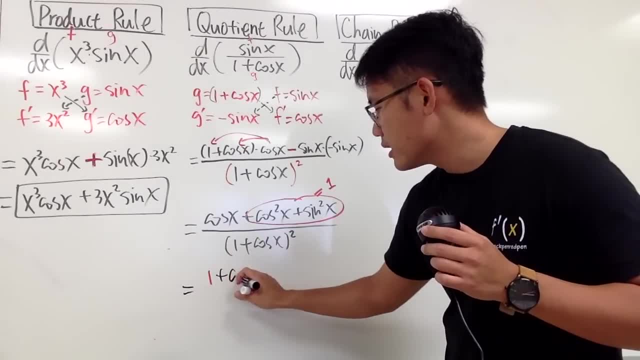 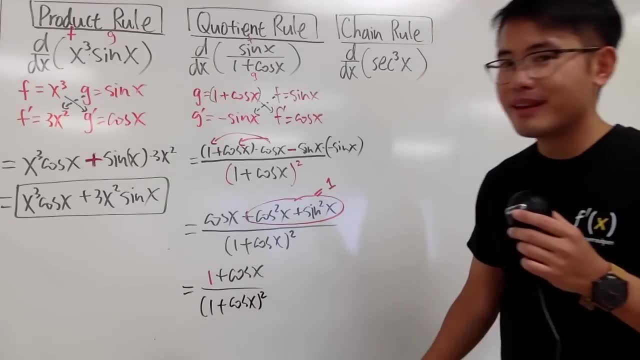 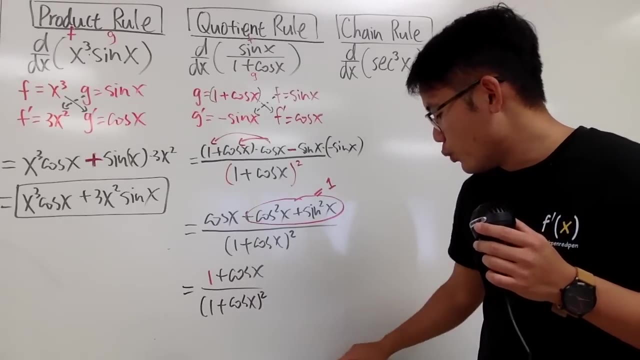 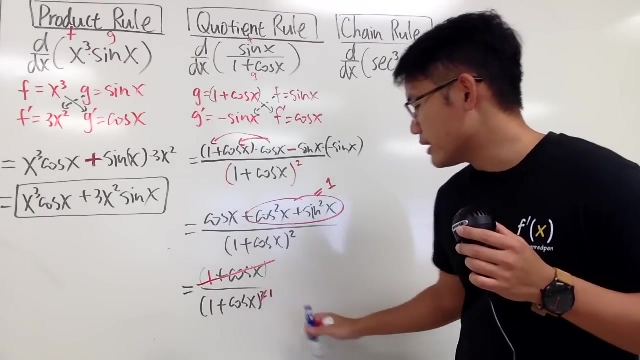 first one plus cosine x, over this one plus cosine x square. and now you see the purpose of me putting down the one right here first. it's because this and that are the same thing. we can cancel one of them out, so let me put on parentheses to be legitimate, i can cancel the top with one of the factors on the. 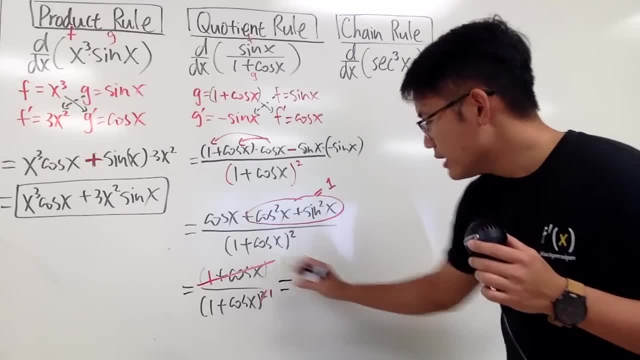 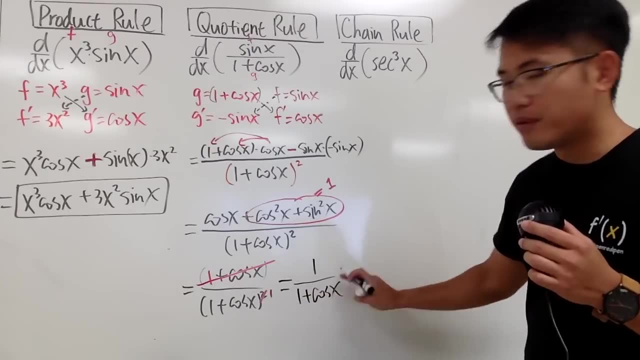 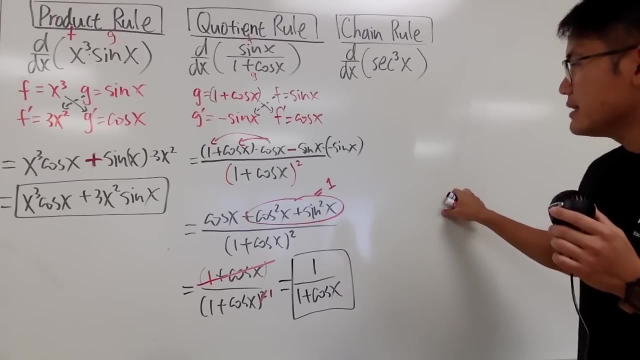 bottom. so in the end we get what? just a one- and this is a nice one- over that, namely one plus cosine x to the first power. so this is all you have to put down and this right here, is it right? and lastly, here's the chain rule, and of course i will have my memory device for you guys right here as well. 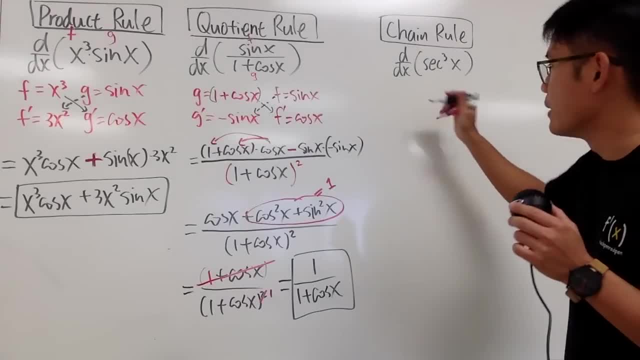 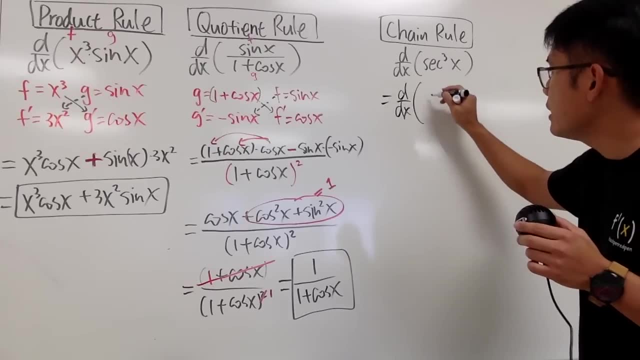 but before we do anything you have to know this notation as follows. this right here is asking you to differentiate when you have secant to the third power. it's the same thing as saying you put parentheses with secant x inside and then raised to the third power. so you can see that this is the 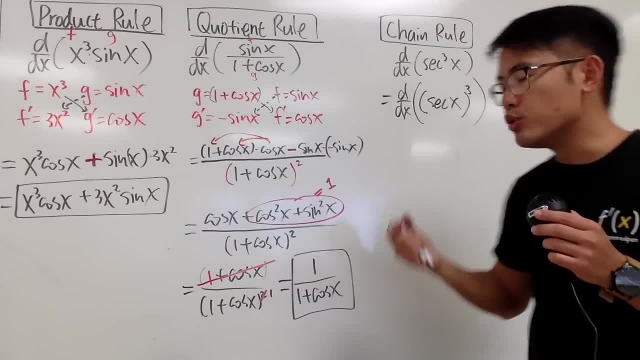 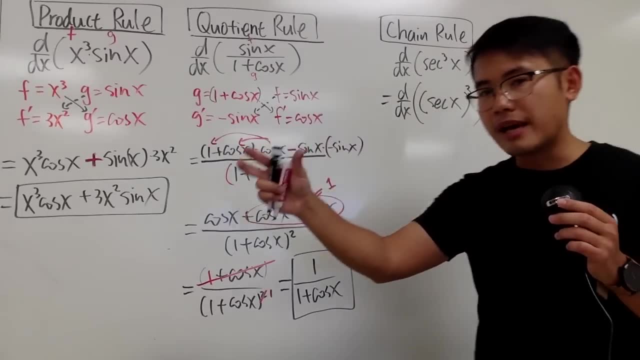 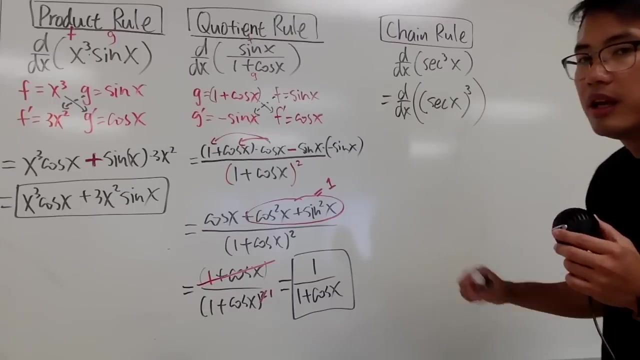 power. when you have powers with trig functions, be sure you use parentheses accordingly. when you have the third power right here, this means you can you take secant x, multiply it three times. so that's what we have. and now here is the deal. you are going to look at this expression and then you 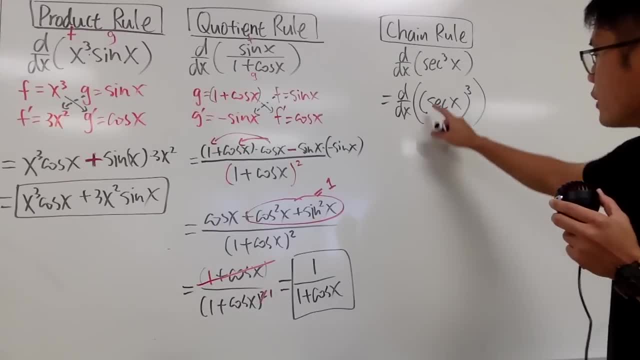 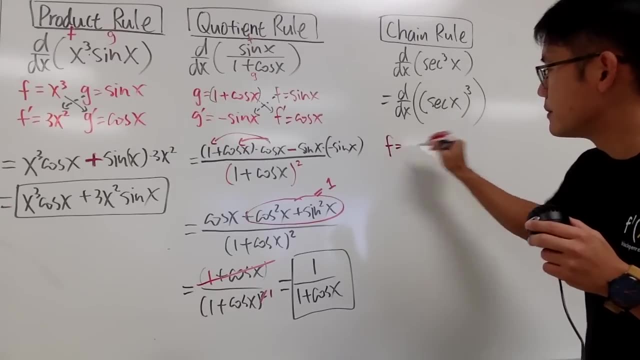 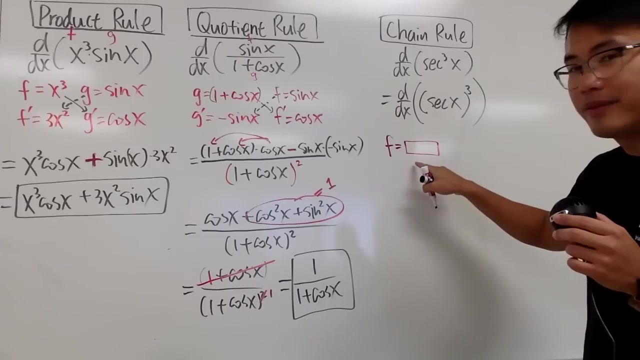 are going to pick up the outer function first. the outer function is: just look at the big picture. you have this to the third power and that's going to be f, and i will label f first. but in this case i'm not going to put down any x for f, but instead i'll put down box right. so we have a box to the. 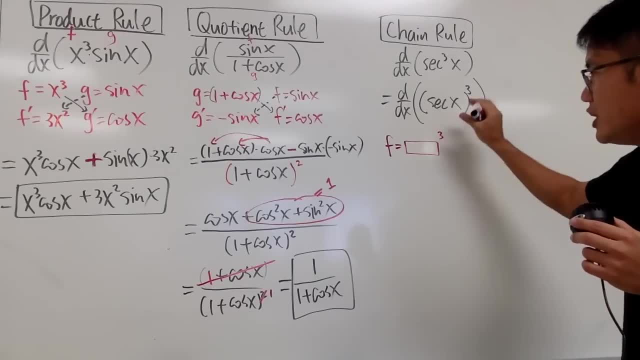 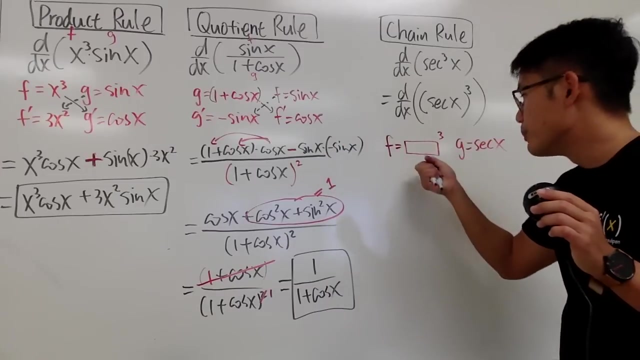 third power like this, and then the g function is what's inside of the box? of course we will have the secant x in the box. so this, right here, is what we have, and now, just like what we have been doing. once we put them down, we can differentiate them individually. 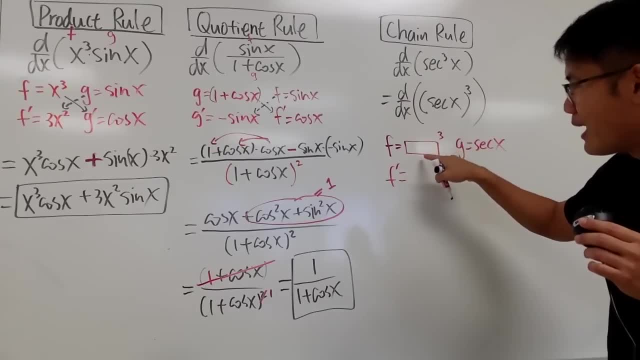 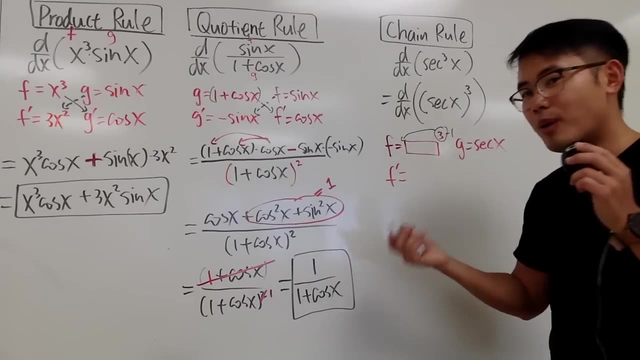 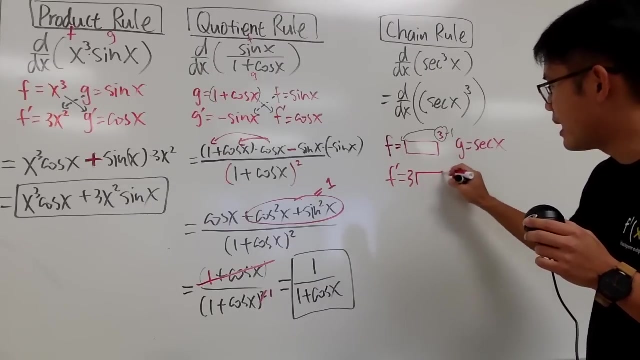 the first one, f prime. this is a box to the third power. so what do we do? well, bring the power to the front and then minus one, the good old power rule right. so we get three. but remember we have a box, so you open the box and then raise that to the second power. anyway, that's pretty much it, seriously. 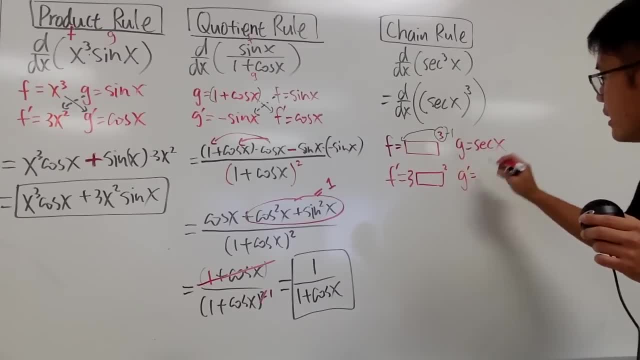 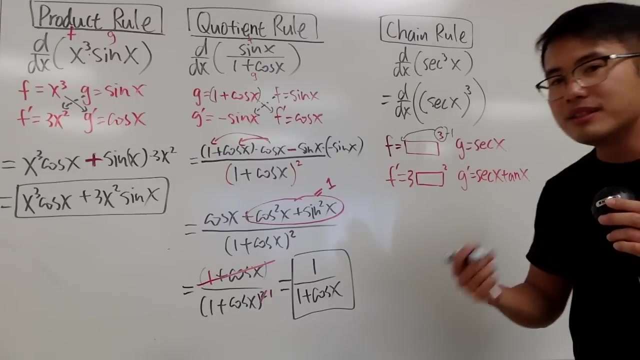 and then look at the g function and, once again, the derivative of secant x. we see that this is secant x times tangent x, and be sure you remember your derivatives, okay. and now this is how you construct your answer for the derivative of secant to a third power. 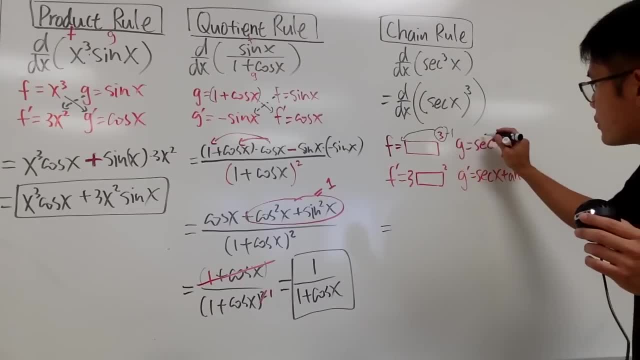 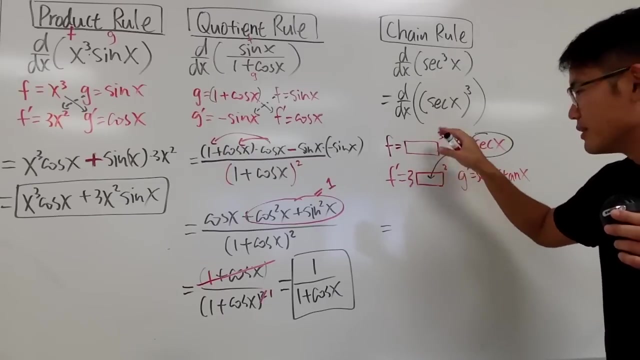 well, this time you are going to look at the g function, which is secant x, and then you are going to put this into the box. okay, and perhaps now let me just erase my circle, because that was just the power rule, to show you the derivative of x to the box, to the third power. 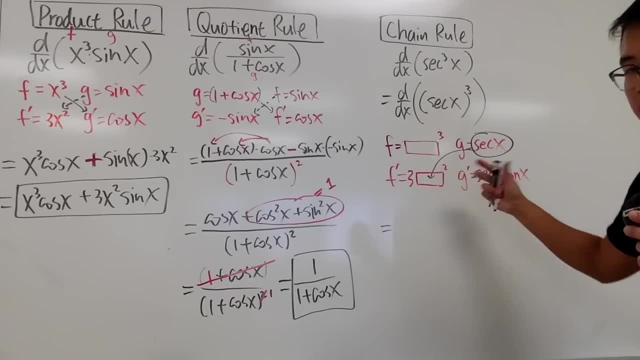 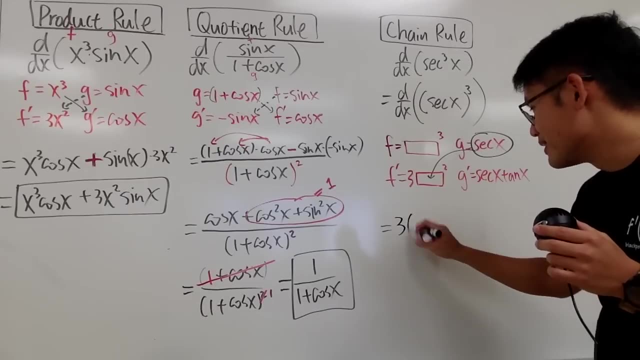 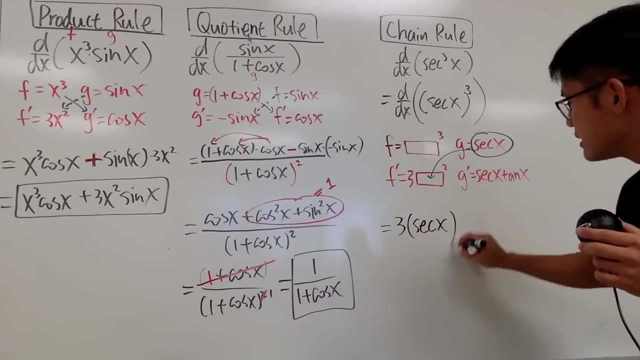 is that, but you put this in the box. okay, this is how you construct the chain rule situation. so we have three, but instead of the box, when you write down the answer, please put down parentheses, okay, so put down parentheses. and then you have the secant x inside and then this is raised to. 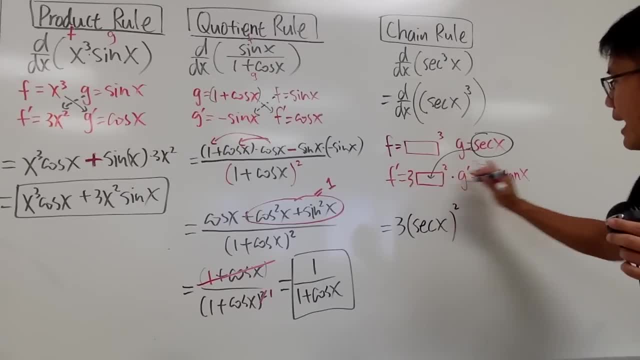 the second power, and then you are going to multiply by this. so just put it down: you multiply by secant x, tangent x, like this. so this, right, here is it. but notice we have secant x to a second power times, secant to the first power, right, so all together you can add the exponents.